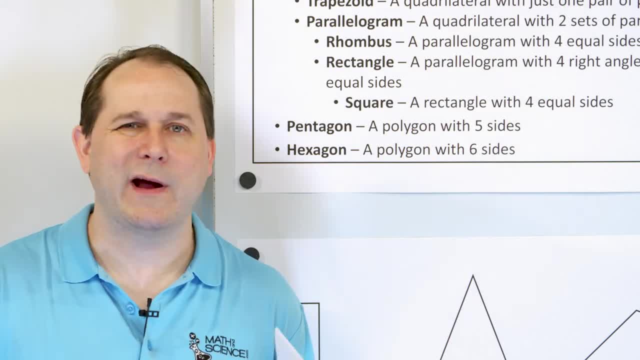 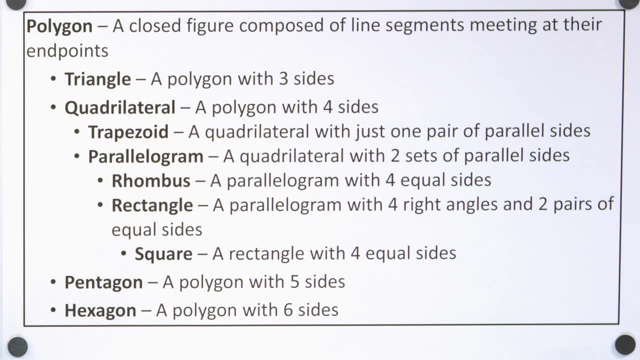 three-sided shape, It's a type of polygon. Any of the square rectangle, any of those quadrilaterals, is a type of polygon. So, under the idea of a polygon, all of these different types, but don't stress out about it, because it's very easy. First of all, 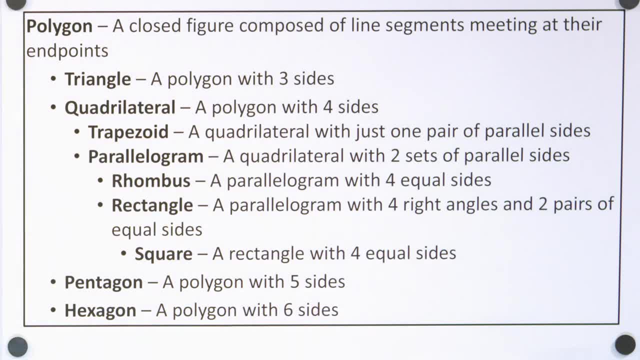 we have a triangle here. It's a polygon with three sides Makes sense Three-sided shape, That's easy, right. Then we have quadrilateral, which is any polygon with four sides. Now let me skip over these, because we've already talked about all of these types of quadrilaterals in the last lesson. 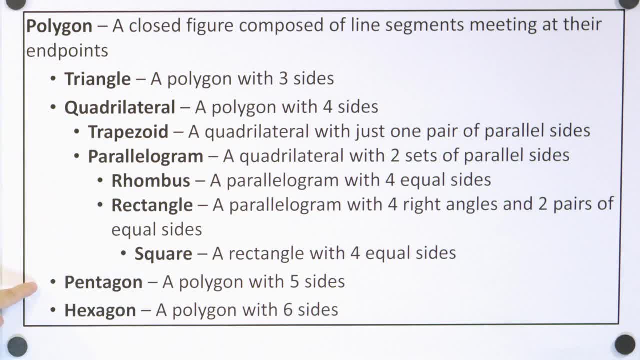 After a three-sided shape and a four-sided shape, we have a five-sided shape, which is a pentagon, and then we have a six-sided shape, which is a hexagon, and then you can go up and down and you can go up and down, and you can go up and down and you can. 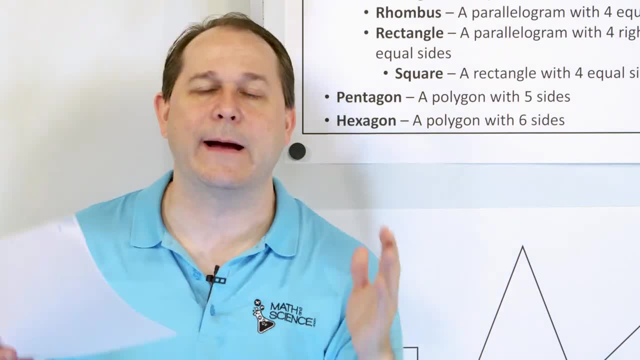 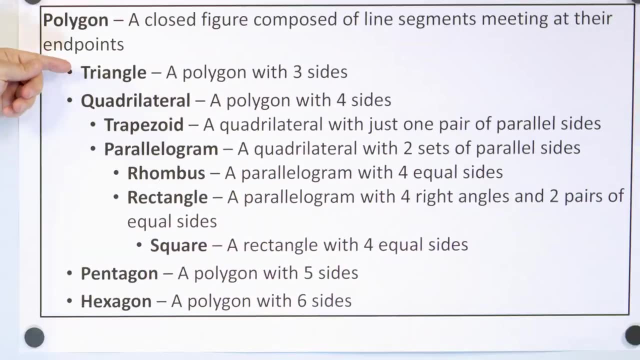 go up from there. For instance, an eight-sided shape is an octagon. You know that's the stop sign shape that we have, So you can have names for all of those different shapes with different sides, but these are the most important ones. So we have a three-sided shape triangle, a four-sided 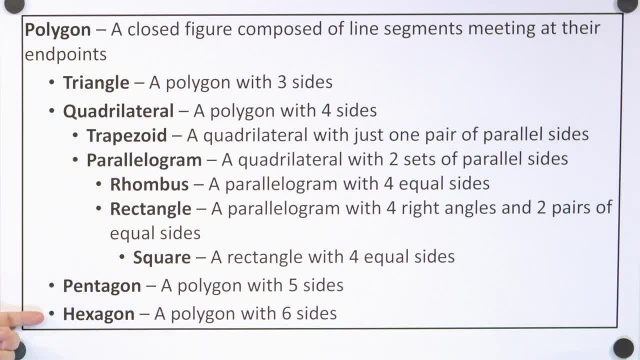 shape- quadrilateral- a five-sided shape- pentagon, a six-sided shape, hexagon, and then, underneath quadrilateral, we have lots of types. We have the trapezoid that we talked about earlier, with only one pair of parallel sides. We have a parallelogram with two sets of parallel sides, but underneath 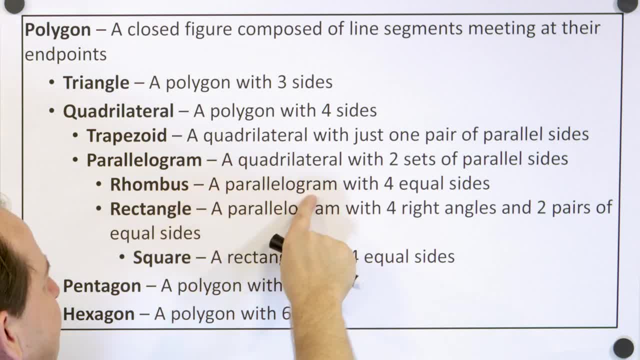 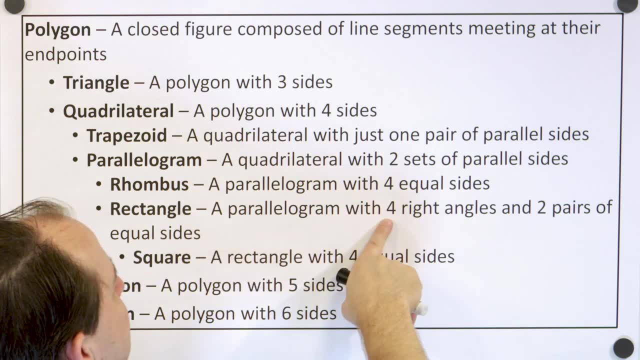 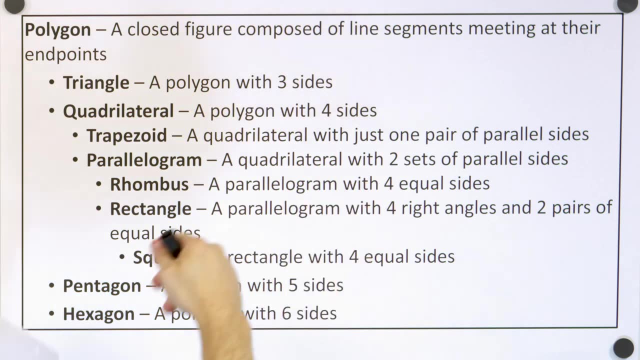 parallelogram. we actually have a rhombus, which is a type of parallelogram where all the sides are equal. We have a rectangle, which is a parallelogram, with four right angles in the corner and then two pairs of equal sides there, So the typical rectangle shape, And then we have a square. 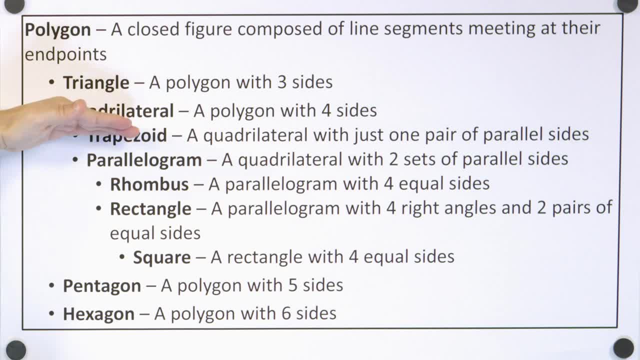 which is a rectangle with all four equal sides. So we've actually studied all of these before. The only thing this lesson is doing is telling us that a polygon is a general thing and we can have three-sided, four-sided, five-sided, six-sided. but I'm also telling you you can have higher sides as well. 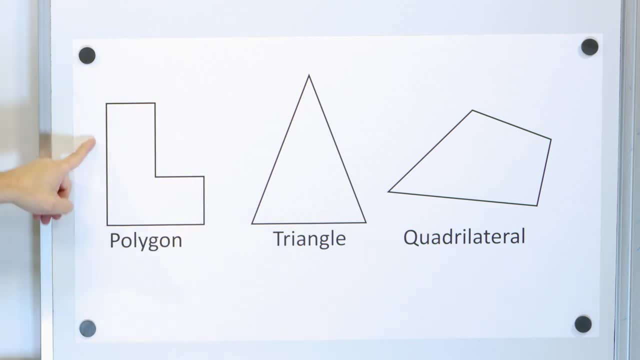 So a polygon is any number of sides with straight line segments connected. Then you have a three-sided shape, We call that a triangle. We have a four-sided shape, We call that a quadrilateral. but inside of the quadrilateral we can have rectangles and squares and trapezoids. We talked about those. 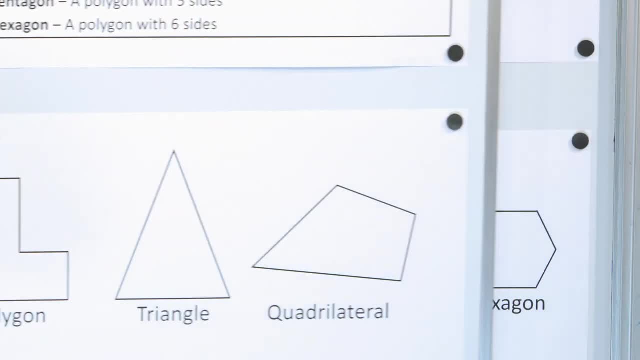 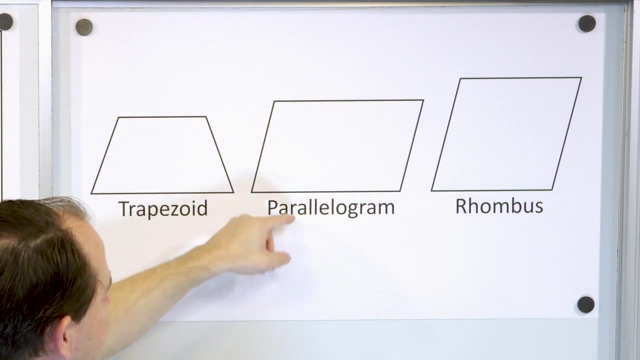 before. So we have three-sided shape, four-sided shape, Then we have a- here's another type of four-sided shape, a trapezoid. Here's another four-sided shape, a quadrilateral. And then we have a three-sided shape- parallelogram. We have opposite sides of that which are parallel, And 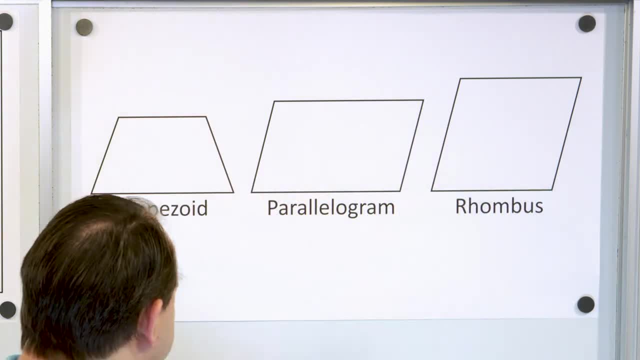 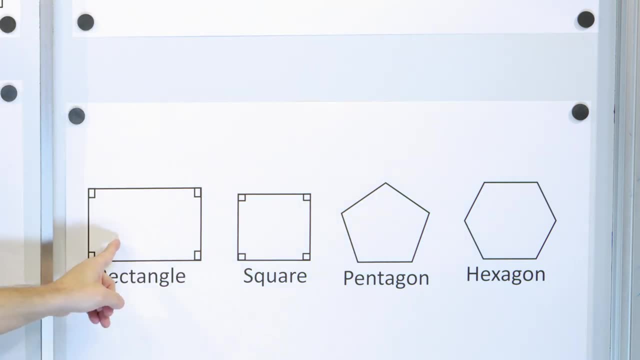 then when we have a parallelogram that has equal length sides, we call it a rhombus, And then when we have a parallelogram like this where all of the angles are right angles in the corner, we call it a rectangle. When we have a rhombus where we have all of the angles in the corner are 90 degree, 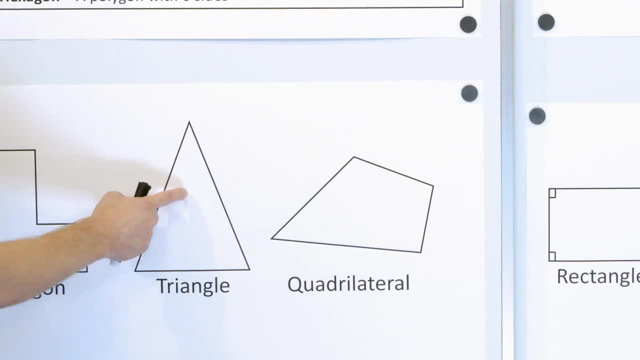 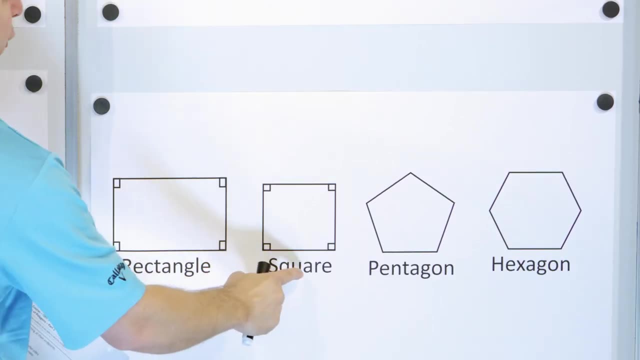 right angle. we call it a square. So you see what's going on here. We have a three-sided shape. Here's the general four-sided shape. All of these trapezoid, parallelogram, rhombus, rectangle, square We've talked about before, those are types of 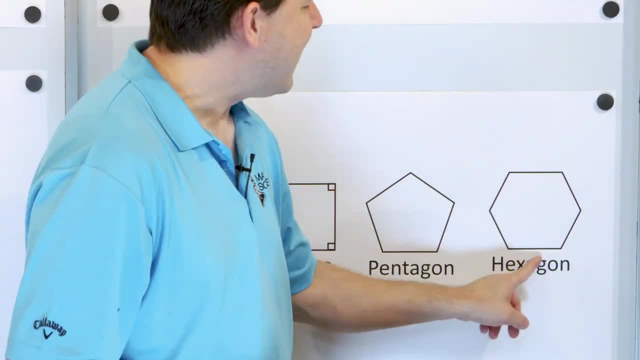 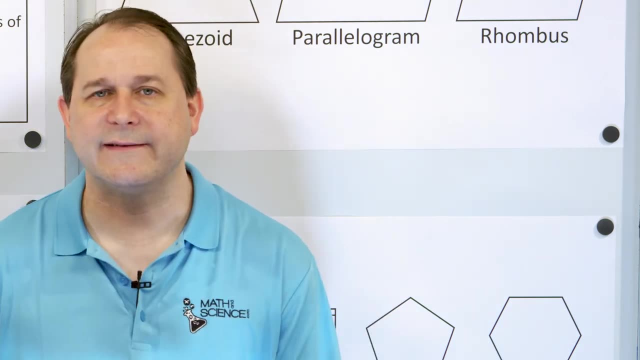 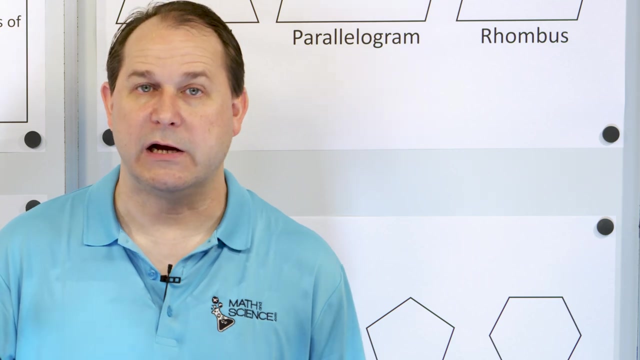 quadrilaterals, And then we have pentagons, And then we have hexagons. One thing I want to talk to you about before we move on is that we have the idea of a regular polygon, or a regular hexagon or a regular octagon, things like that. A regular polygon is a polygon where all of the sides are. 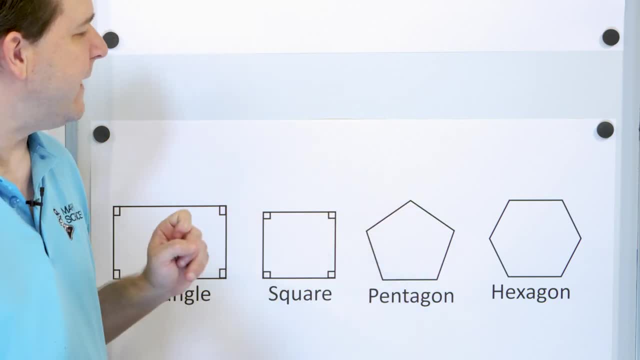 the same length and all of the angles on the inside are the same measure, Because I can draw different kinds of pentagons. I can draw different kinds of pentagons. I can draw different kinds of hexagons. All I need is a five-sided shape. It doesn't have to look beautiful like this: I can draw. different kinds of hexagons, that are six-sided shapes, that are all weird shapes. But when we say we have a regular hexagon, then all of the sides have to be the same length and all of these inside angles have to be the same angle. Regular means nice and symmetric, basically All the sides. 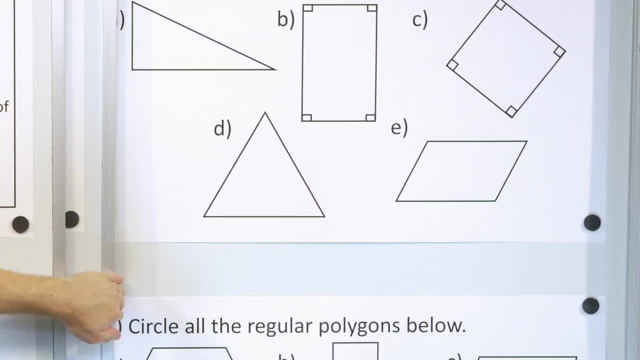 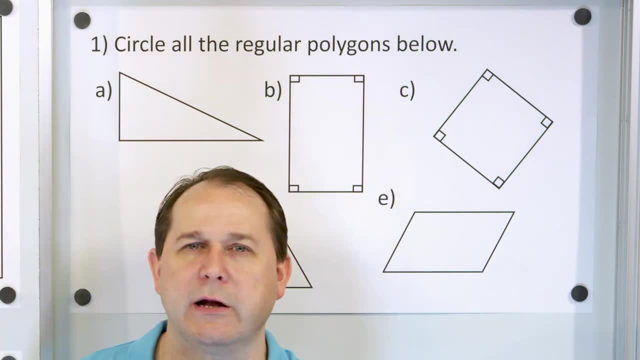 are the same. All of the lengths and the angles are the same as well. So here's our first problem. It says circle all of the regular polygons below. Regular regular polygons means all of the sides have to be the same length and all of the inside angles have to be the same. So this is a triangle. 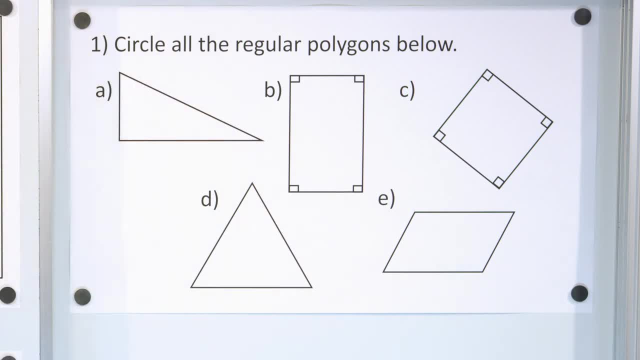 and that is a polygon. but it's not a regular polygon because the inside angles are not the same and the triangle length, the sides are not the same. This one is a regular polygon because the inside angles are the same and the outside edges are all the same length as well, So I can. 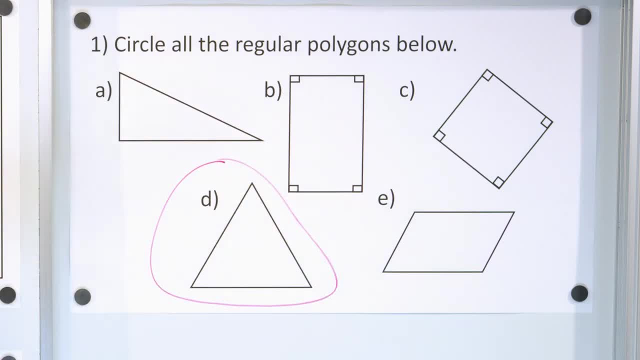 circle. this one That's a regular triangle, or also called a regular polygon. Alright, what about this one? The sides are not the same length, so it's not a regular figure. What about this one? The sides are not the same length, it's not a regular figure, and also the angles are not. 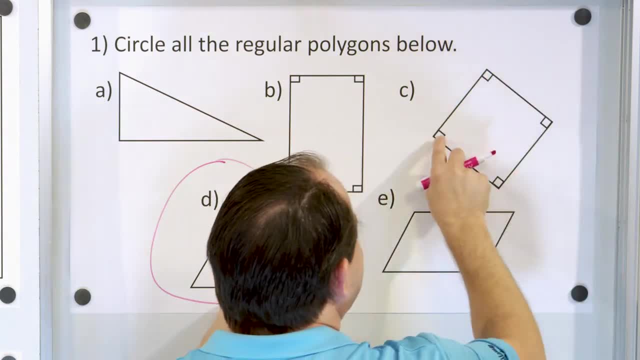 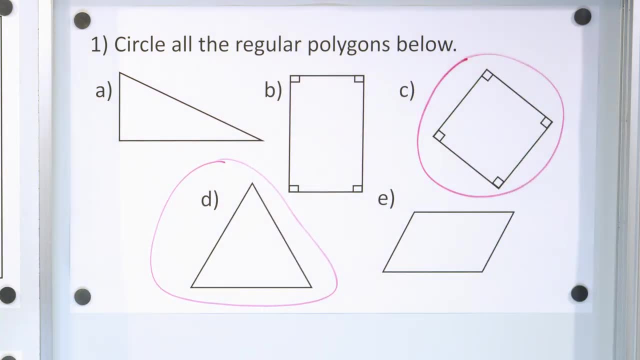 the same as well. What about this one? Well, the sides are all the same length and the inside angles are all the same as well, so we call that a regular. it's a regular polygon. We also call it a square. Alright, let's take a look at problem number two. 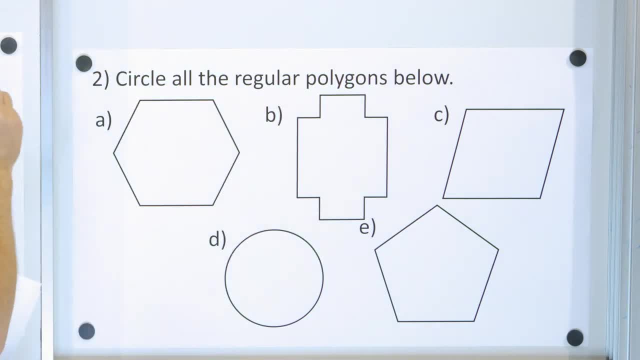 Let's circle all of the regular polygons here. Remember, all the sides have to be the same length, all of the angles have to be the same. Which ones are regular to you? Well, we have one, two, three, four, five, six- we call that a hexagon- and all the sides 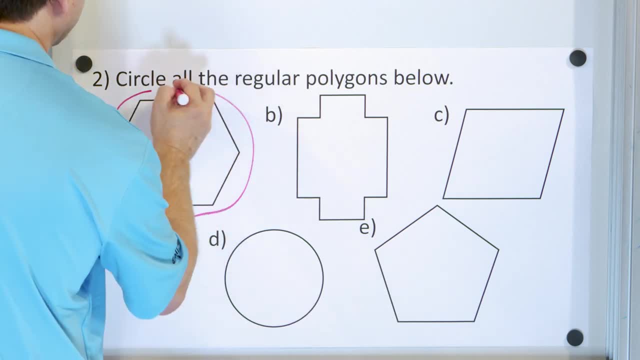 are the same length, all of the angles are the same, so this is a regular hexagon or a regular polygon. What about this one? The sides are the same length, but the angles are not the same, so that's not right. What about this one? 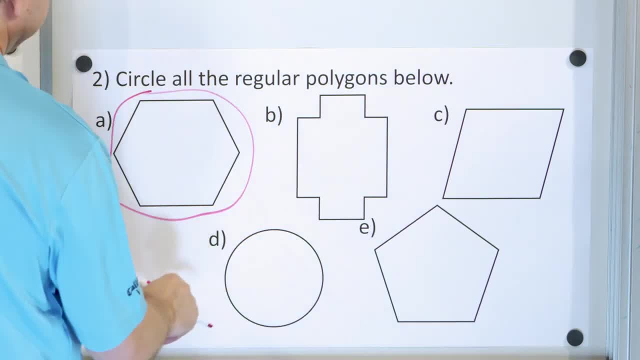 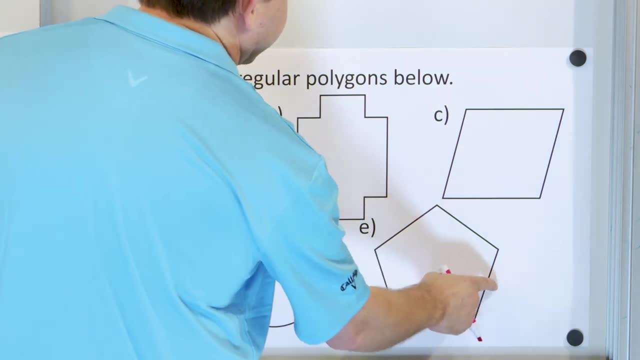 The sides are not all the same length, so that's not right. What about this one one? Well, a circle is not a polygon at all, So that one doesn't count. What about this one? We have here a pentagon. One, two, three, four, five. Remember, pentagon is five-sided shape. 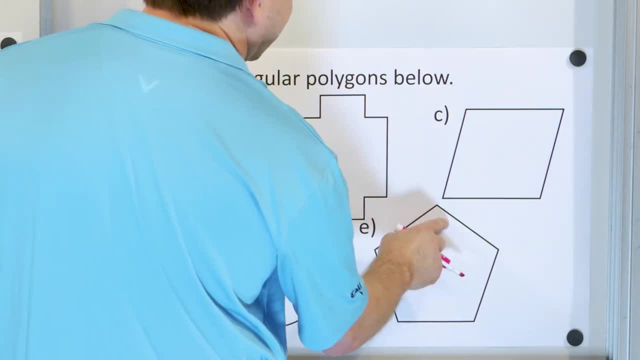 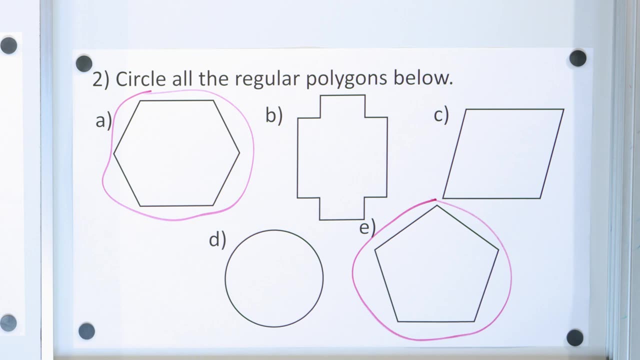 Is it regular? All of the lengths of the sides are the same and all the angles are the same. So we're going to call this a regular pentagon. So those are the two shapes that are here that are regular. These are regular because the sides are the same length and the angles inside are the 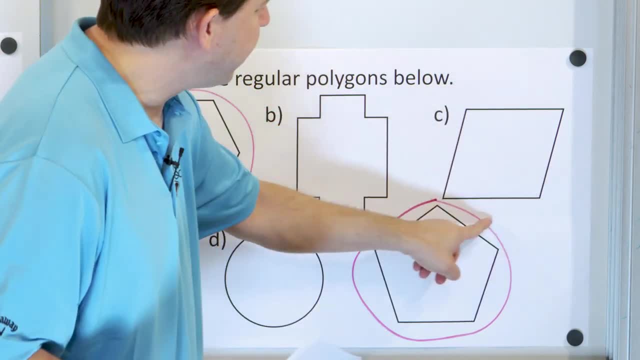 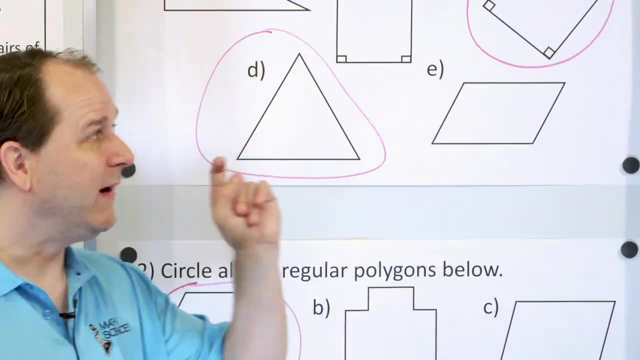 same. This is a polygon, but it's not a regular polygon. This is also a polygon, but it's not a regular polygon. And this one here, a circle, it's not a polygon at all, because polygon what It has. 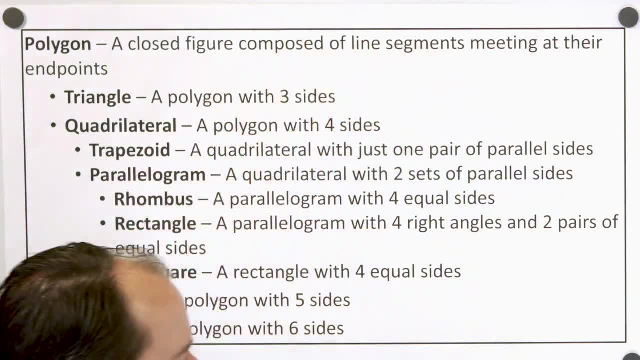 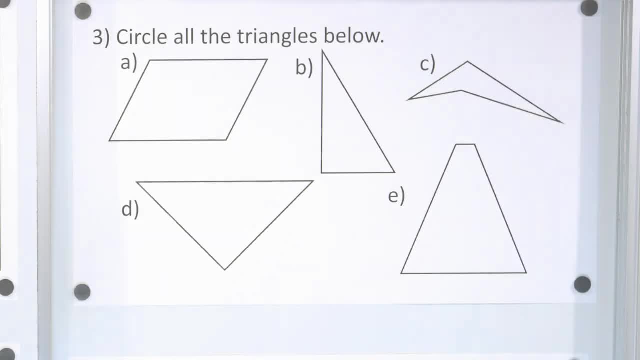 to be a shape composed of line segments. But a circle, of course, is not a shape that is composed of line segments. So let me take these down. I have two more problems to talk about with you. Problem number three: circle all the triangles. Triangle is what? A three-sided closed figure. 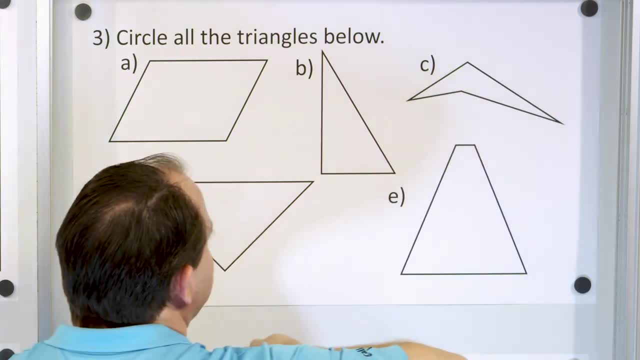 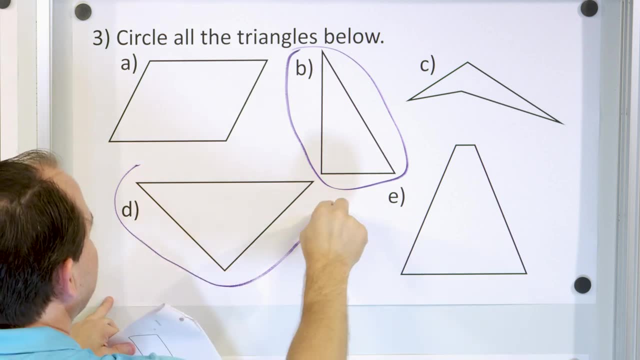 So this is not a triangle, It's a quadrilateral. We have four sides there. Here's a three-sided shape, So obviously this is a triangle. Here is a three-sided shape, So obviously it is a triangle. Notice, we didn't ask for the regular.